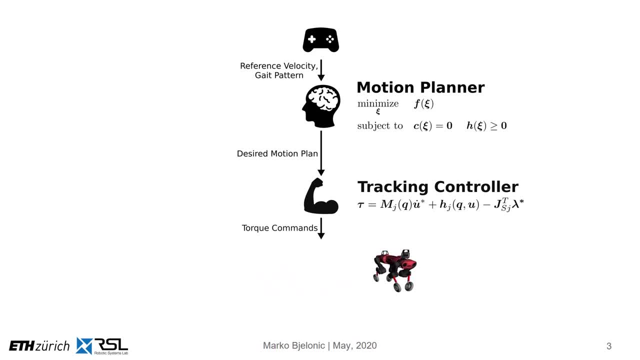 plan. we are presenting a novel whole body controller that is able to track these trajectories by sending torque commands to the real robot. First I am describing the motion planner that splits the problem into wheel and base trajectory optimization. By splitting up the problem, we are able to solve the optimization in real time on the robot and in a model predictive. 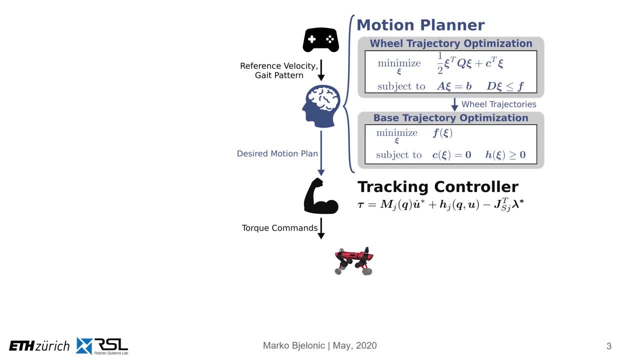 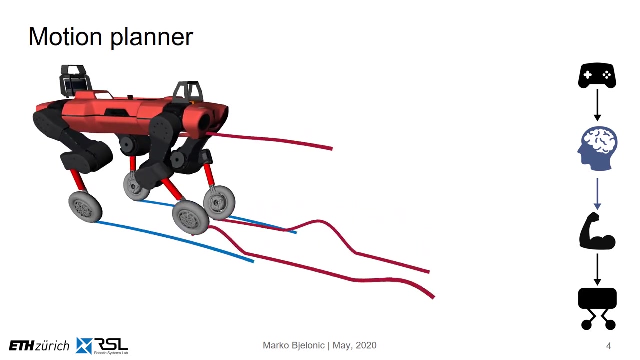 control fashion. The wheel trajectory optimization is minimizing some quadratic cost that is subjected to some linear equality and inequality constraints. Given these trajectories, the base trajectory optimization solves the nonlinear problem as described before. As shown in this animation, we are interested to find feasible trajectories of the base. 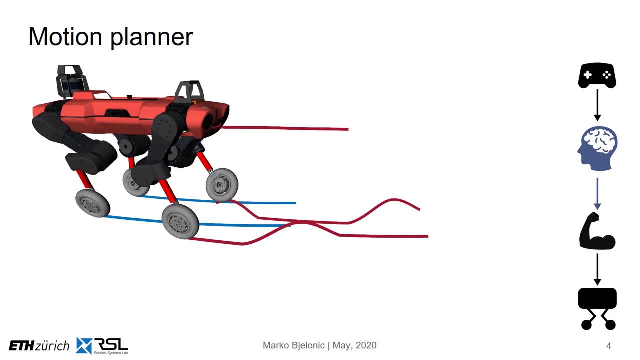 and all four wheels over a predefined time horizon into the future. The motion planner optimizes over the center of mass position, velocity and acceleration. Similarly, we would like to find the equivalent orientations and its derivatives at each point in time. Moreover, the trajectory of each wheel needs to be determined. 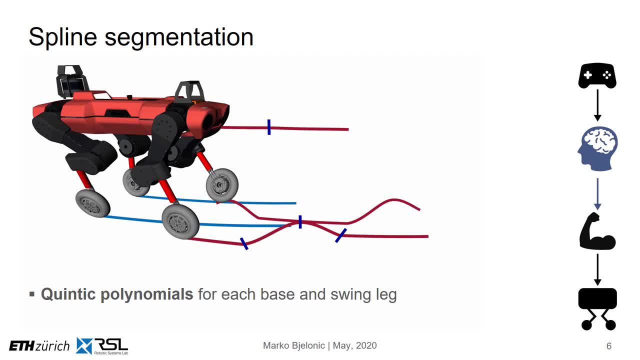 We are accomplishing this by segmenting the trajectories into several splines, where we define quintic polynomials for each base and swing leg. Contrary, we are defining the motions on the ground as a quadratic polynomial for each velocity, which then inherently captures the rolling constraints on the ground. 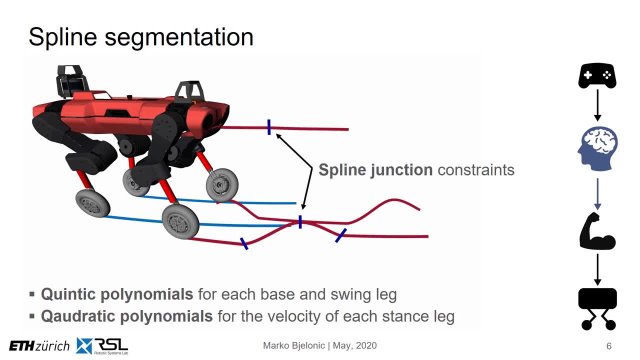 To connect each of these polynomials, we define junction constraints between them. The trajectories start at each start of the optimization with the measured state of the robot wheel, which are given by the onboard sensor readings. Moreover, at the end of the time horizon, we fix the final condition of the center of. 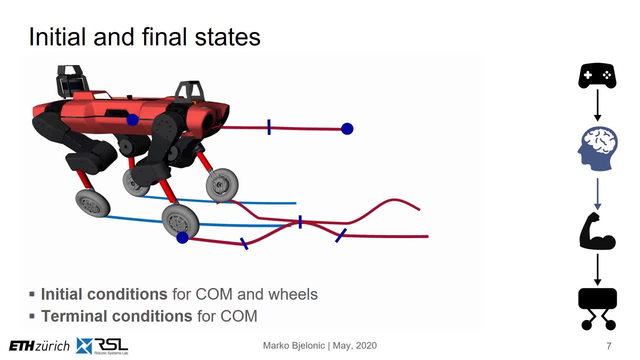 mass which is given by the joystick commands or the high-level planner To generate smooth motions. we minimize the accelerations of the trajectories. We are avoiding leg extensions by adding inequality constraints that define the maximum range of moved leg and add a small cost that guides the wheel to a projected tip position on the 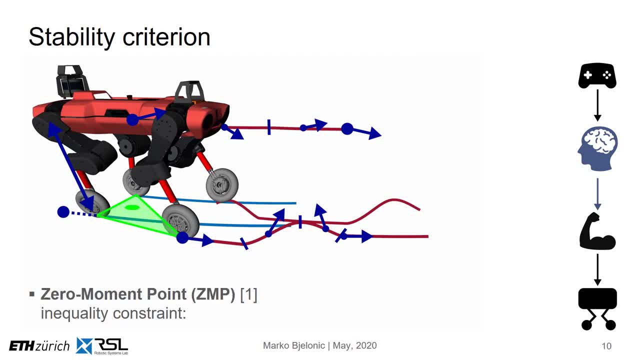 ground. We also define a stability criteria for 밀q. The amount of delegates is estimated at the random line and spaced mix. idolgo is based on the idea of the zero moment point and we generalize this approach for weird legged robots. The zero moment point as defined here, is a function of the gravity inertia forces that are. 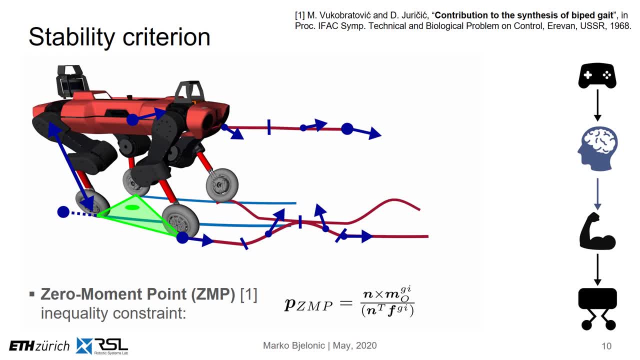 acting on the torso of the robot. More specifically, this point needs to be inside the support polygon, which is spanned by the legs on the ground. Here we show the example of a support polygon in the form of a green triangle, since three legs are in contact with the ground. 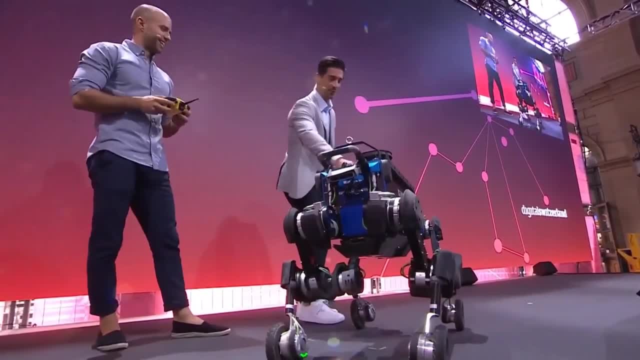 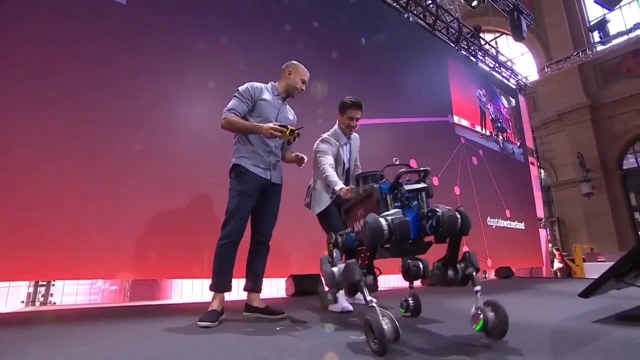 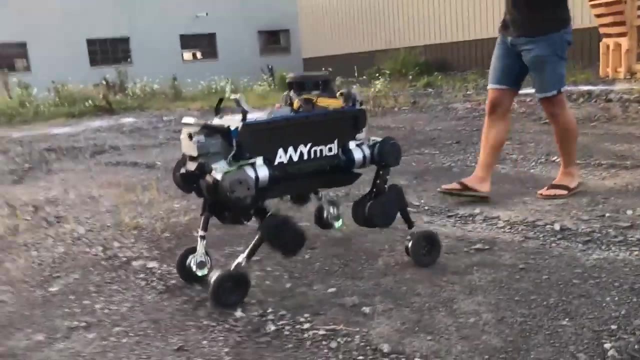 Having everything in place, we are able to create stable motions, as shown here. The robot is able to withstand external forces by generating reactive motions. In addition, the robot is able to deal with rough terrain, as shown here in this gravel pit. On top of that, we are able to create several hybrid gaiters. The robot is also able to move around the ground in the form of a green triangle, since three legs are in contact with the ground. Having everything in place, we are able to create stable motions, as shown here in this gravel pit. On top of that, we are able to create: 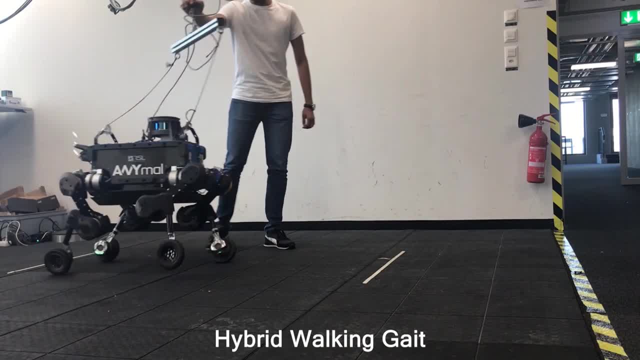 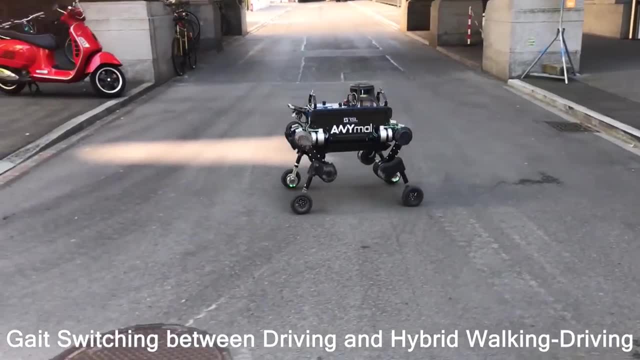 several hybrid gaiters. The robot is also able to move around the ground in the form of a green triangle with different gait timings, like a flying trot, walking gait or pacing gaits. More importantly, we are able to switch between driving and walking gaits when needed. So the robot is able to drive. 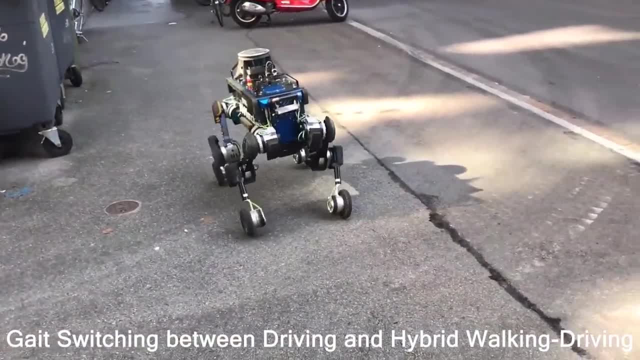 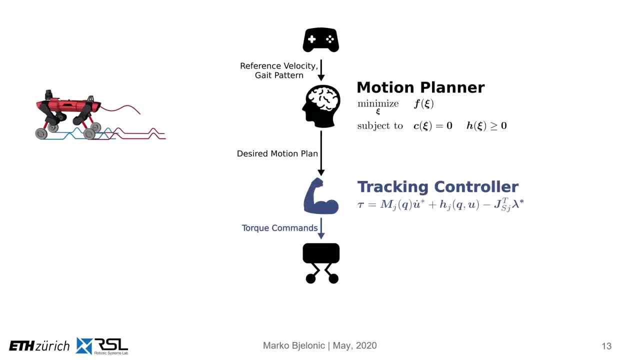 on flat terrain and, whenever it is needed, the robot switches to any walking gait that is able to overcome challenging obstacles. Given these trajectories, the next question is how are we able to train the robot to drive on flat terrain and whenever it is needed, the robot switches to any 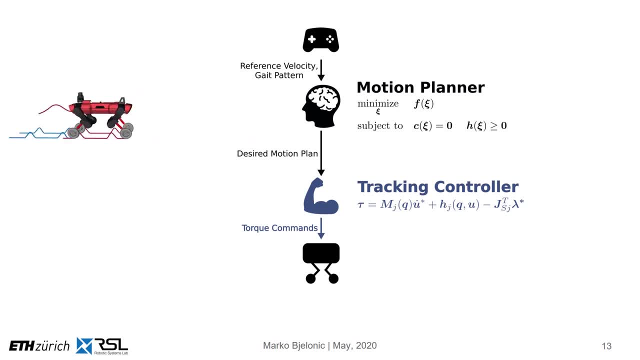 driving gait that is able to drive on flat terrain? Does it require initial training and fast dusting? And, more specifically, how are we able to send commands to the robot? The real robot consists of 60 motors that need to be coordinated to achieve such kind of highly dynamic motions. 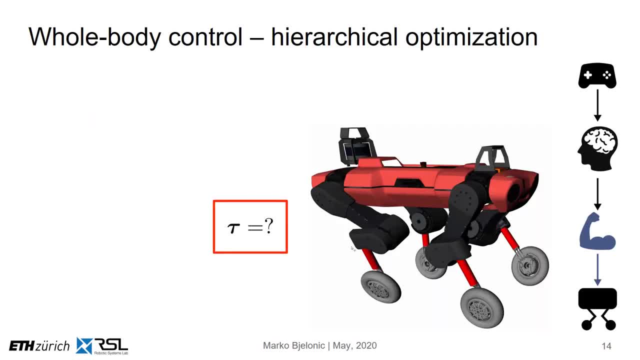 What we are really concerned about is to generate the vector tau, which captures all the 16 joint torques that are later sent to the real robot, And for this we are using the whole body controller, which is based on a hierarchical optimization We are solving 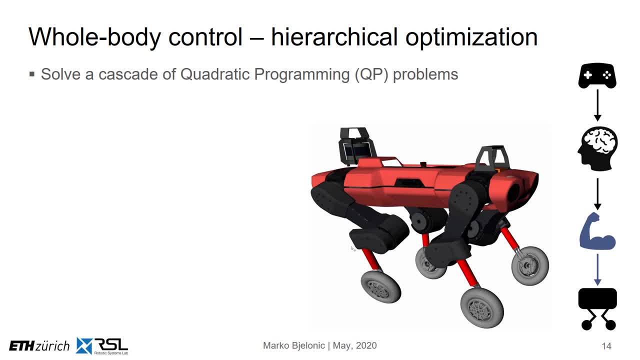 a cascade of quadratic programming problems where we optimize over generalized accelerations, u, dot and contact forces. lambda. We describe the dynamics of the robot with equality and inequality constraints that are here defined as tasks. so how do tasks look like? So, for example, a task could be some. 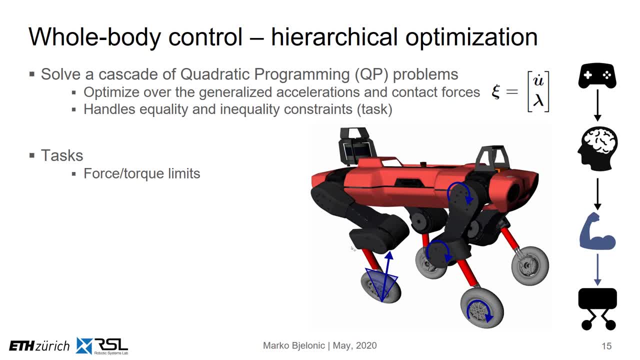 force or torque inequality constraints. As shown in this image, the ground reaction forces need to respect the friction constraints but at the same time the generated torque cannot be higher than the maximum torque of each motor. The rolling constraints defines that the centripetal accelerations on 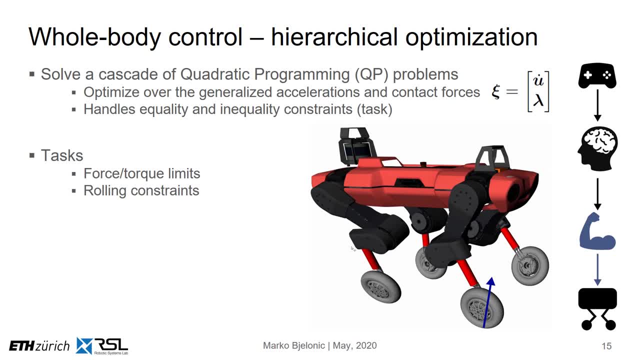 the robot are less than the torque of each motor. At the same time, the the ground needs to be a vector that point towards the center of the wheel. We might want to minimize all contact forces to reduce ambiguity And, in a similar fashion, we are able to define more tasks. 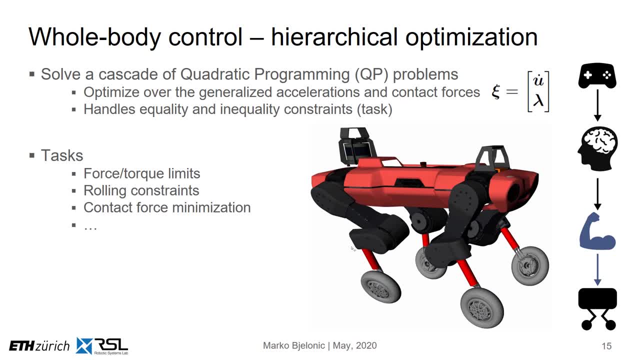 Given the optimized generalized acceleration u dot star and contact forces, lambda star, we plug these entities into the equations of motions as shown here. Here, m is the mass matrix, h captures all non-linear terms which are given by Coriolis and centrifugal terms. 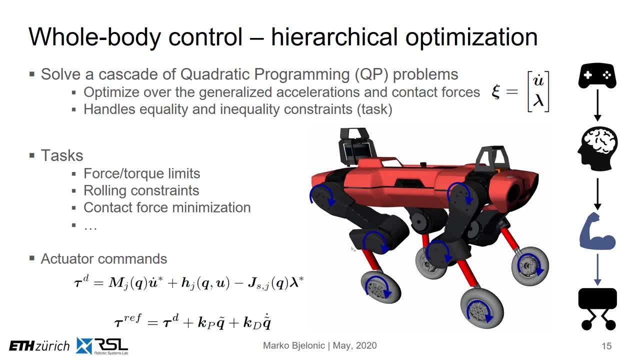 And the optimized contact forces, lambda star, are transformed by j into the space of joint torques tau. Finally, we send these desired joint torques tau d as a feed forward signal to each of the drives And in addition we add PD gains on top of that to be robust against muddle uncertainties. 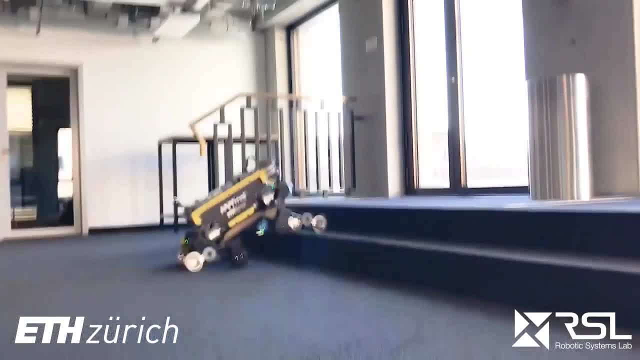 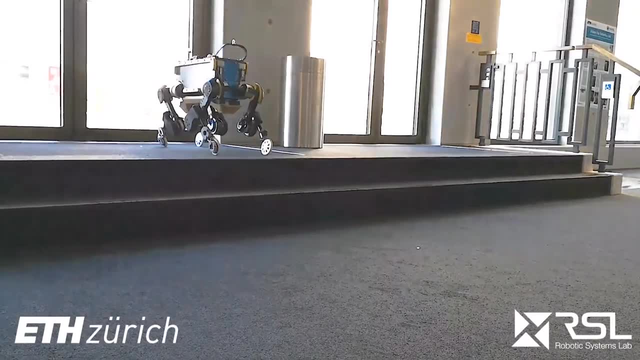 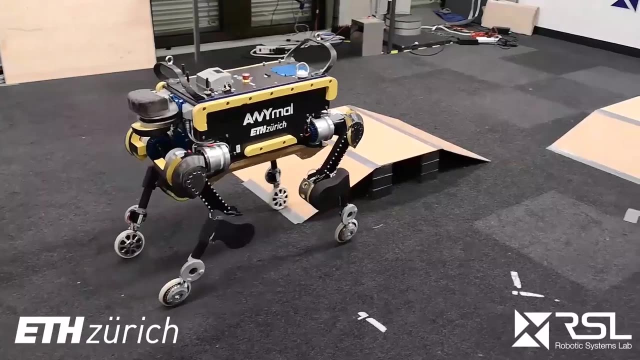 This video shows nicely the benefits of our force control approach. We are able to create smooth motions. The robot here has no idea about this set of stairs, but because we are using a torque control approach, the robot is able to adapt to this unseen terrain. 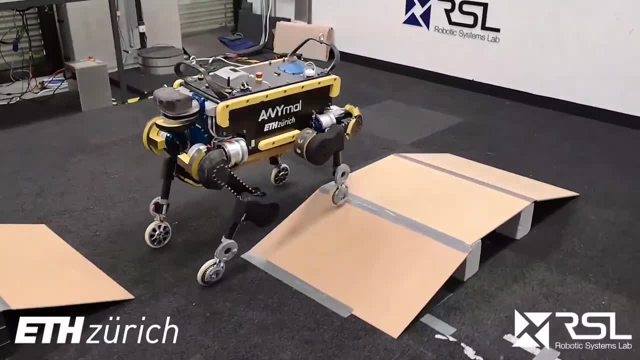 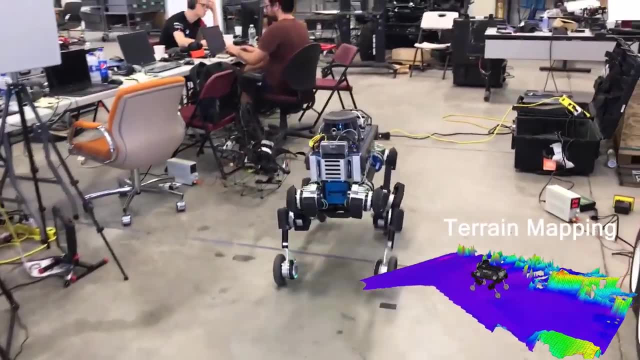 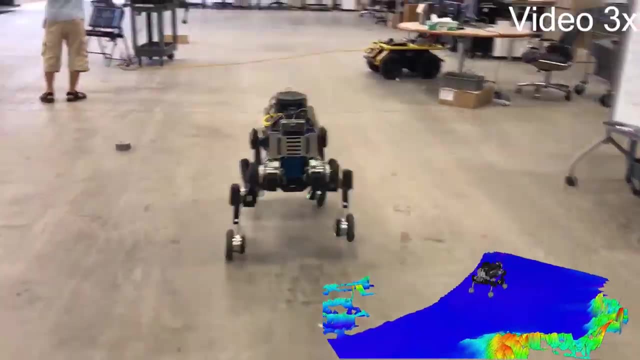 Again, the robot is locomoting here blindly over these inclines. Putting everything together, we are able to run a complete mission Here. the robot is mapping the environment in front of him. as shown in the lower right, The robot is able to detect objects, as, for example, this backpack, and report its position.